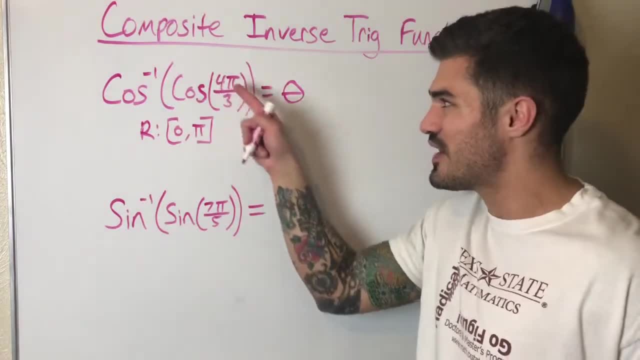 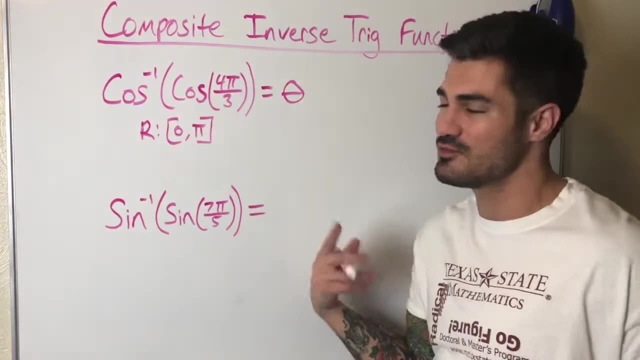 because that's what inverse functions do, right? They take in a value and spit out an angle, Basically the opposite of regular functions, which take in an angle and spit out a value. So it makes sense, right. So I'm still looking for an angle. 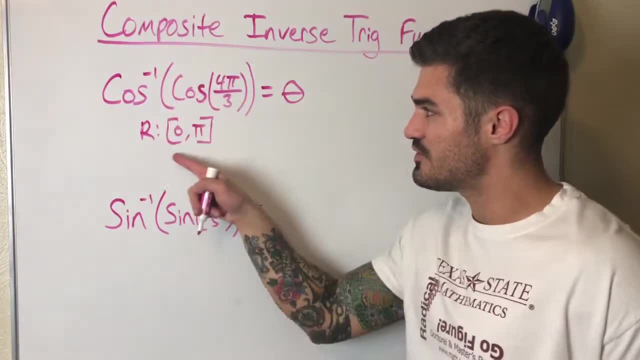 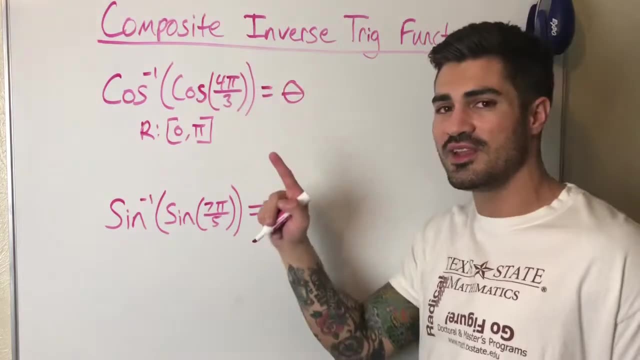 but 4 pi over 3 is not within the range of cosine inverse, So I need to find a different angle that is within the range. So how can I do this? Well, luckily for this example, I know what cosine of 4 pi over 3 is. 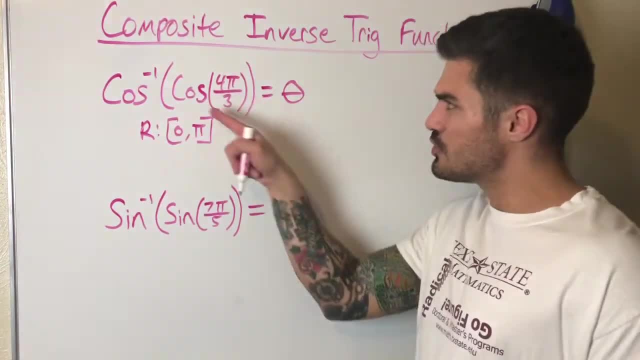 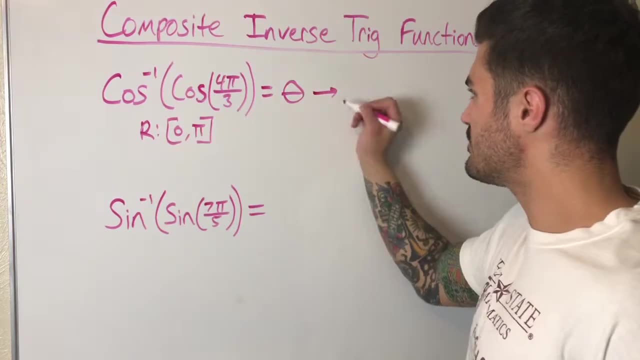 It's actually on the unit circle and I can find it. So I can replace cosine 4, pi over 3 with what it equals and then I can evaluate this. This is one of the more straightforward examples. Most of them will not be like this, right. 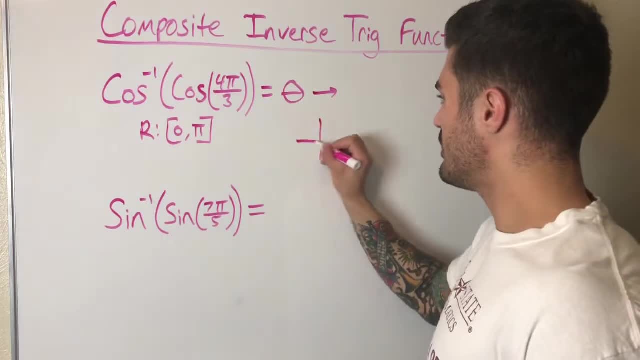 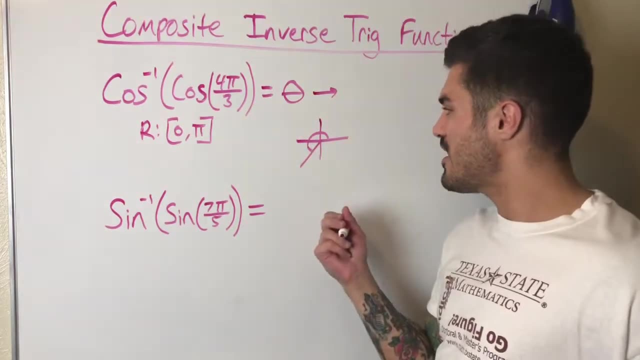 So what is cosine of 4 pi over 3?? I don't have the unit circle memorized, but I know that 4 pi over 3 is in the third quadrant. I know that the reference angle is pi over 3, so it's going to be one half. 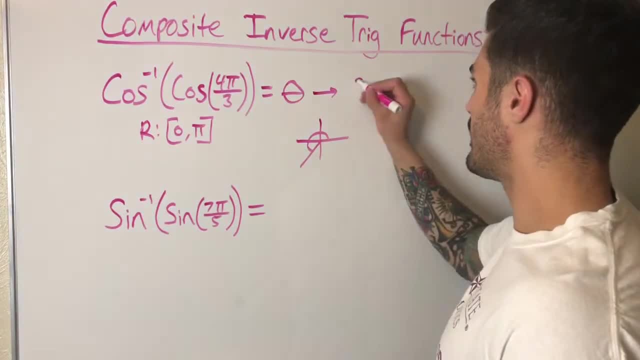 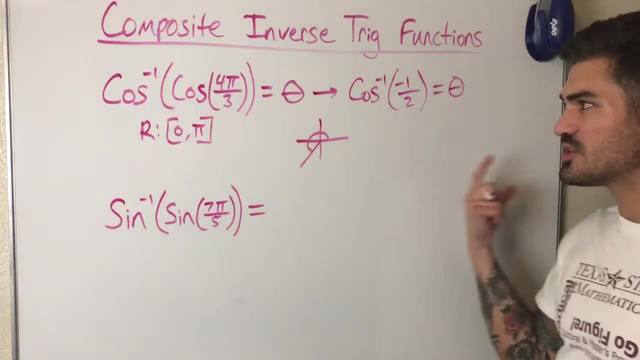 but it's in the third quadrant so it's going to be negative. So we have negative one half. So cosine inverse of negative one half equals theta. And now, hopefully this looks a little more familiar- We can switch theta and negative one half. 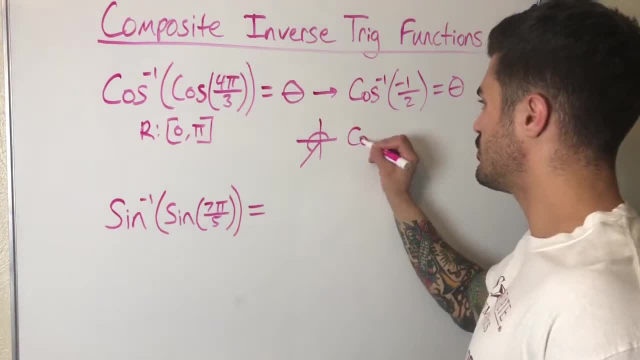 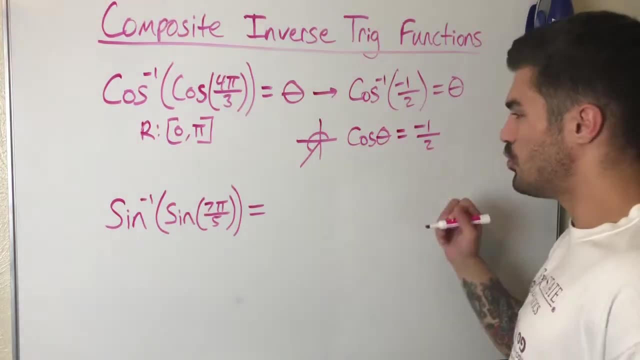 and write this as not an inverse function, right? It is just cosine, right? This is like saying, cosine of what angle gives me negative one half. But what's specific about this angle? Again, it has to be within this range. It has to be between zero and pi. 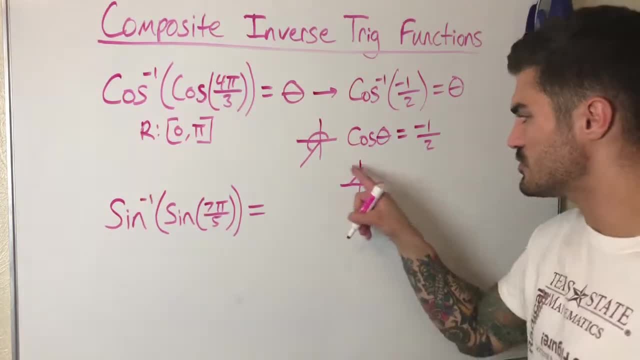 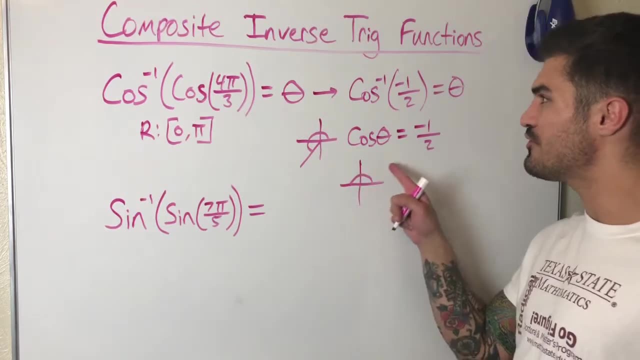 So, if I draw a little picture here, I'm dealing with zero to pi, so first or second quadrant. Since I have a negative, I know it's going to be second quadrant. So I'm in the second quadrant and I have a reference angle of pi over 3.. 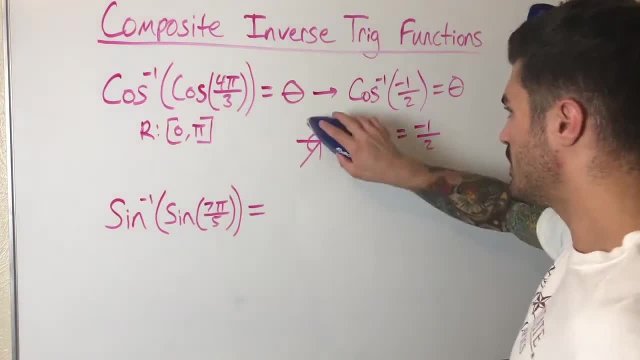 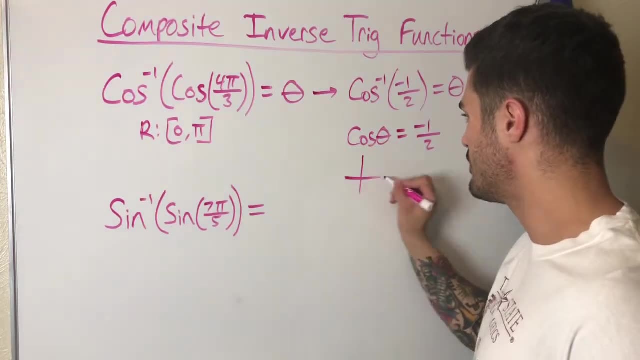 So if I let's see, I should redraw this. Pictures are. the key to a lot of these is drawing pictures. I highly recommend it. I do not do any of these examples without drawing a picture ever, So draw this. So again, I'm looking at a reference angle here. 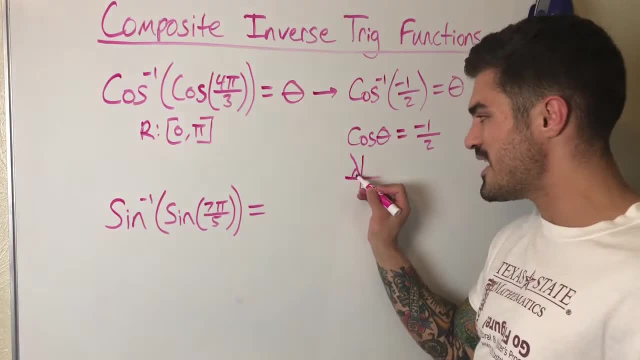 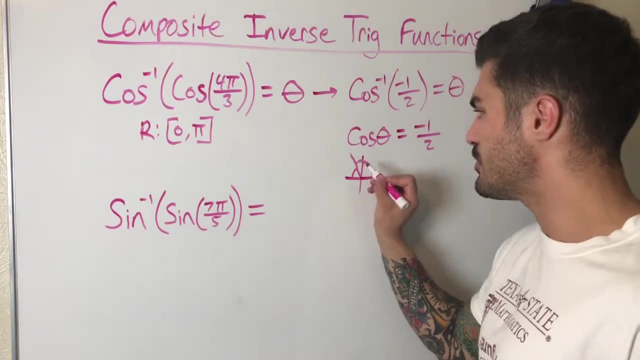 of pi over 3.. So that means the angle between the x-axis and the terminal side of my angle is pi over 3.. That means the angle between the initial side, like the actual angle itself I'm looking for, is 2 pi over 3, right. 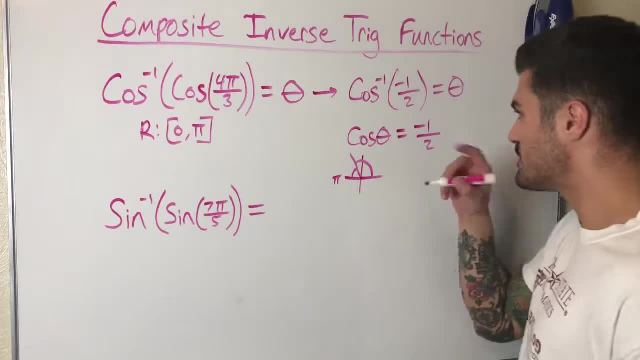 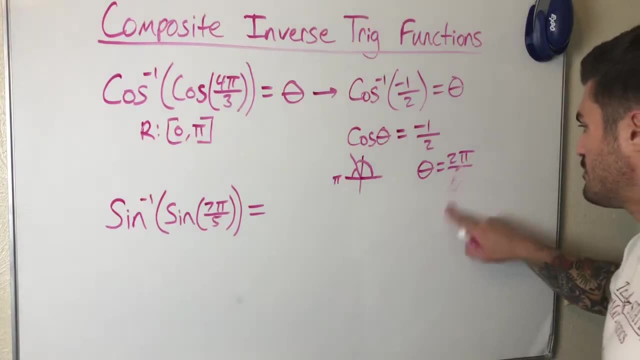 Because this is pi. I basically take pi and subtract pi over 3.. So my theta in this case is 2 pi over 3, which whoops 2 pi over 3, which I can confirm is within the range I'm looking for. 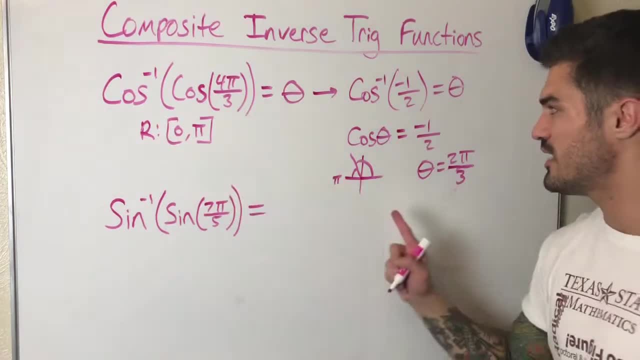 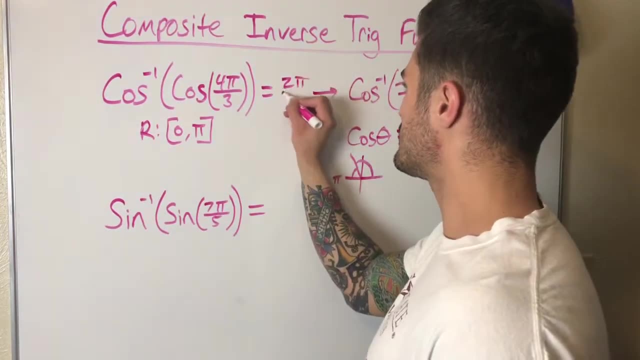 2 pi over 3 is definitely between 0 and pi and it definitely gives me negative 1 half for cosine. So the solution to this is 2 pi over 3.. Hopefully that makes sense. All right, so now let's look at this example. 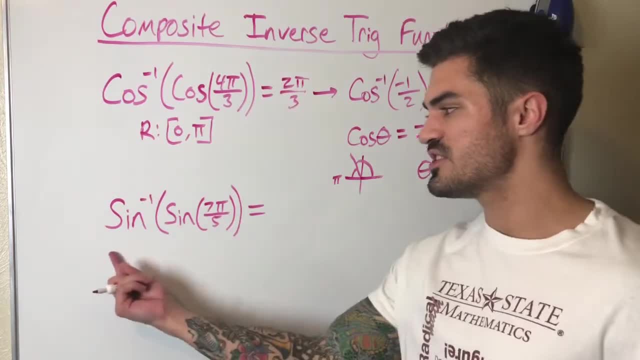 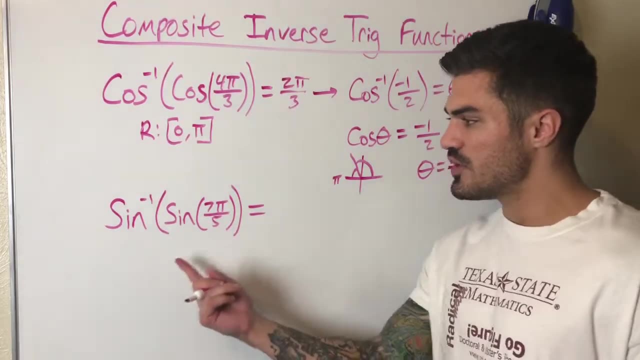 Our inner function is sine of 7 pi over 5. Outer function is sine, inverse. So again, we have to first check because if you look at this angle and you see that it is within the range of our outer function, our inverse function, 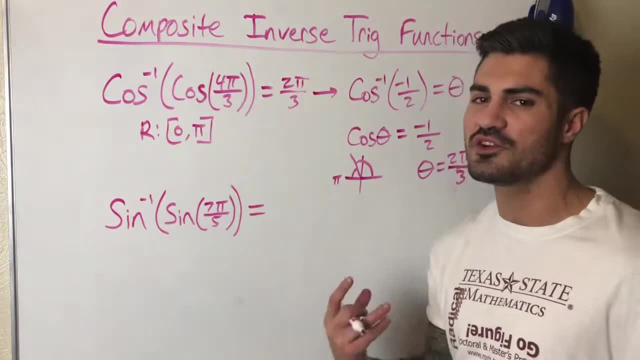 then you can just cross out, cross out, write that as your answer, right? So that's the first step you usually always want to take is double check, see if it is within that range, cross those out and that's your answer. 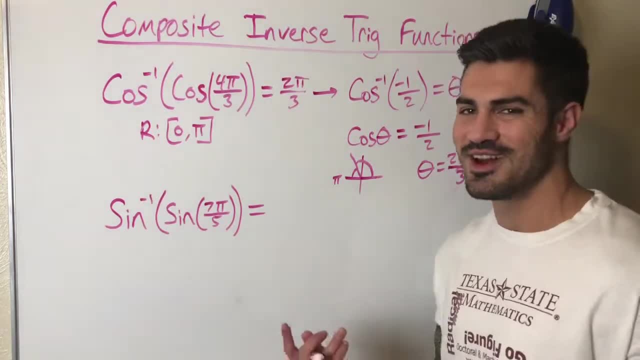 But it's usually not going to be because the instructors want you to know what to do when it's not. So it's probably not, and in this case it isn't. because what is the range of sine inverse? It is from negative pi over 2.. 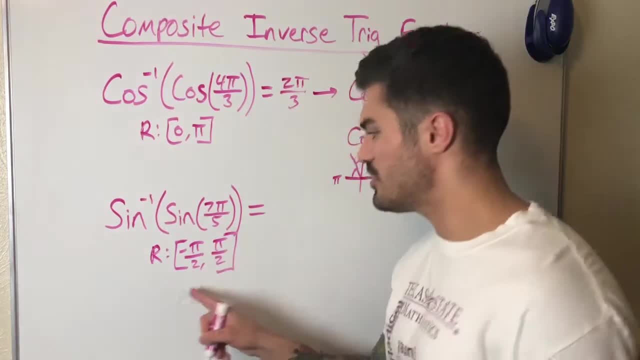 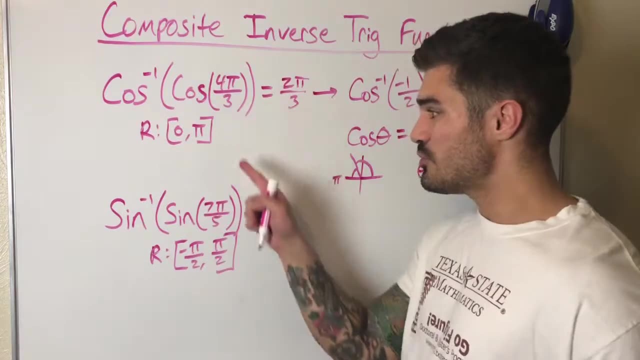 To pi over 2,. okay, From negative pi over 2 to pi over 2, this is clearly bigger than pi over 2.. It is not within the range. So what do we do? Well, in this example, we looked on the unit circle. 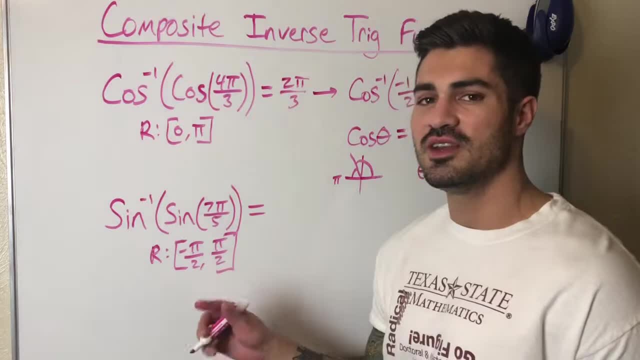 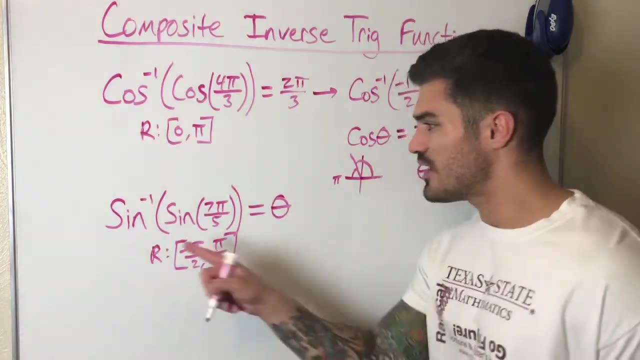 but in this example we do not know what sine of 7 pi over 5 is. I have no way of finding that out without a calculator, so we have to do something different. So I know that this is going to be theta right. 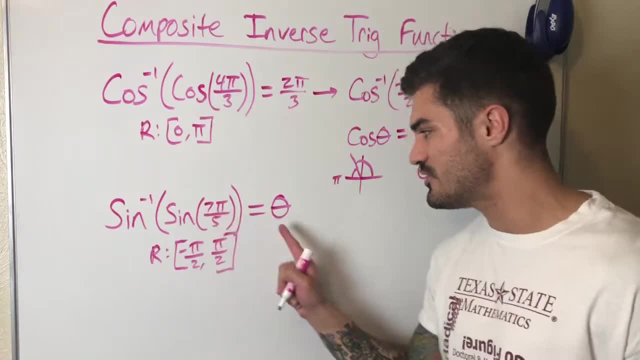 I'm still looking for an angle, because I have an inverse function. This is some value. It's spitting out some angle. That's how sine inverse works. So I'm looking for some angle. So couldn't I just do this step here? 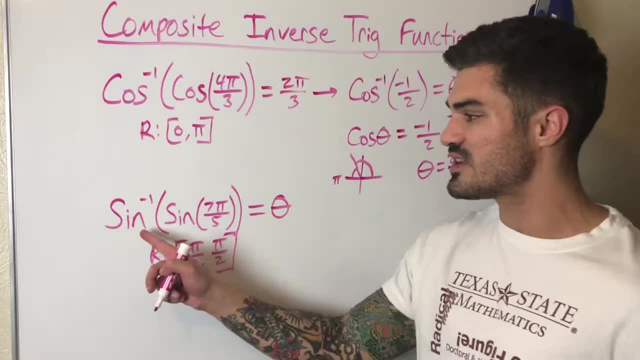 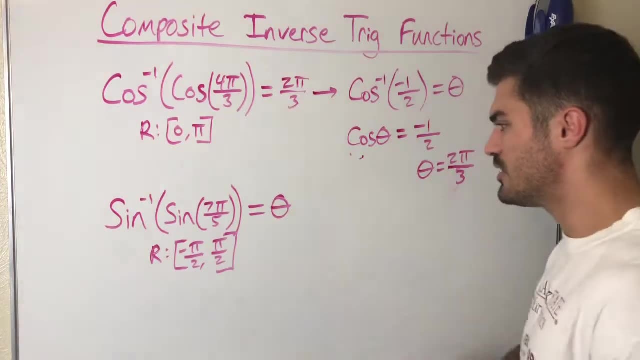 Couldn't I do this step. This is still some value. I could still say. this is like saying: sine of what angle equals sine of 7 pi over 5.. So that's exactly what I'm going to do in this next step, and I've got to make a little room here. 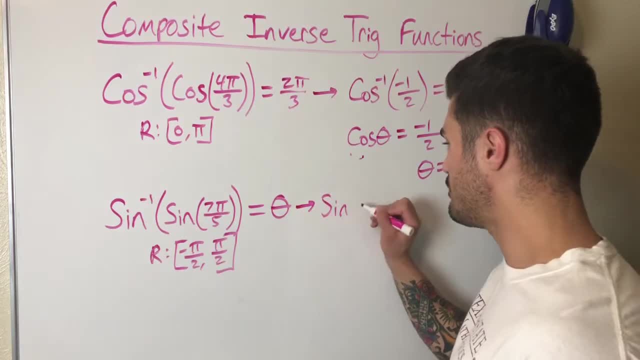 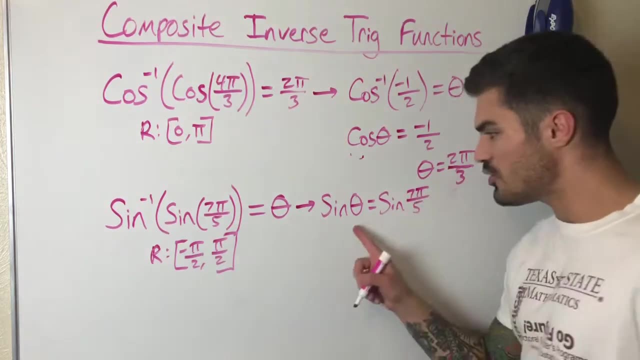 So that's exactly what I'm going to do. I'm going to rewrite this as sine of what angle equals sine of 7 pi over 5.. This angle has to be within negative pi over 2 and pi over 2.. It has to be within that range. 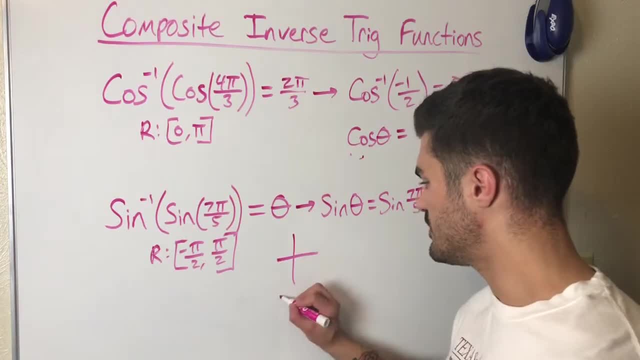 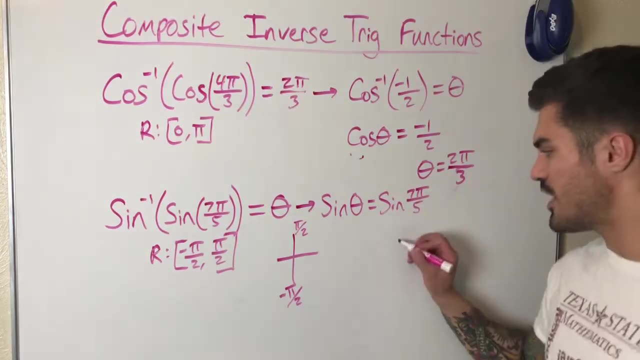 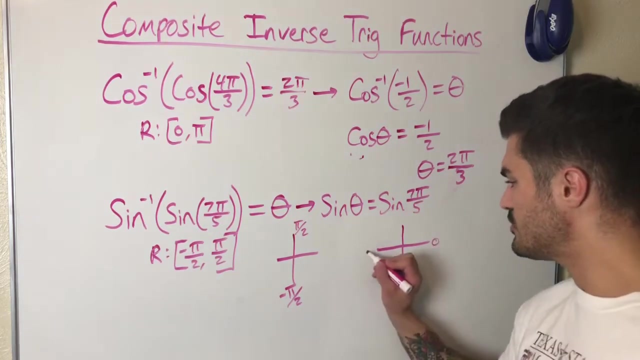 Okay, So this angle I'm looking for is between negative pi over 2 and pi over 2.. Okay, So let me draw 7 pi over 5.. 7 pi over 5 is where It is in the third quadrant, because we're going from 0 to pi. 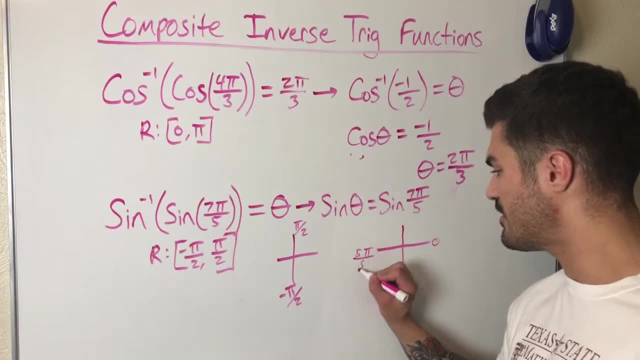 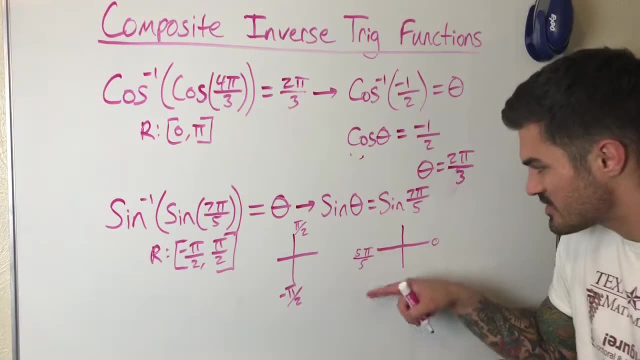 I can rewrite pi, if that makes more sense, as 5 pi over 5.. Some people like having that common denominator, because then I can see that this is 2 pi over 5 past 5 pi over 5.. So this angle: 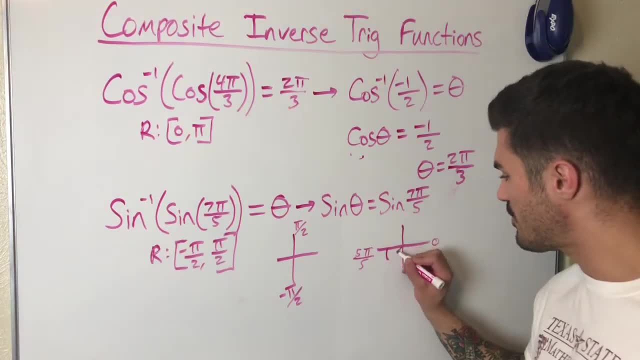 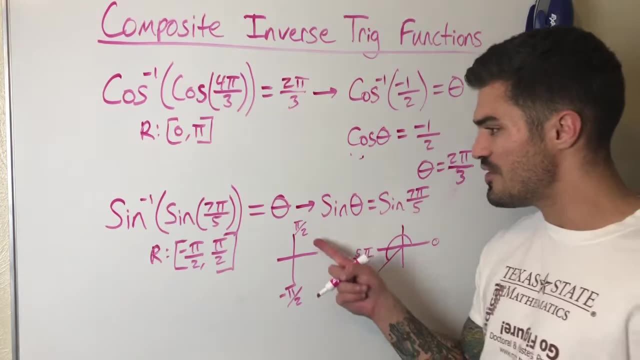 which happens to be the reference angle, is 2 pi over 5.. The full angle is 7 pi over 5.. So I'm looking for a value within the range of sine inverse, which is from negative pi over 2 to pi over 2,. 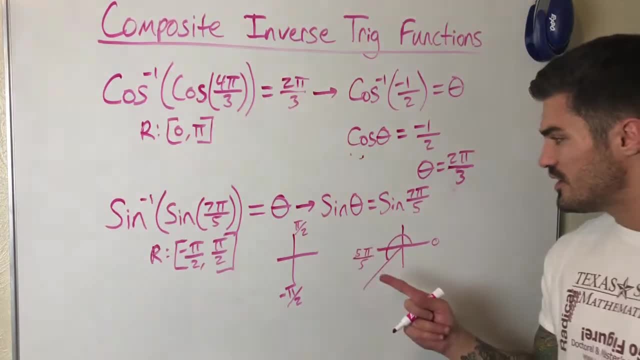 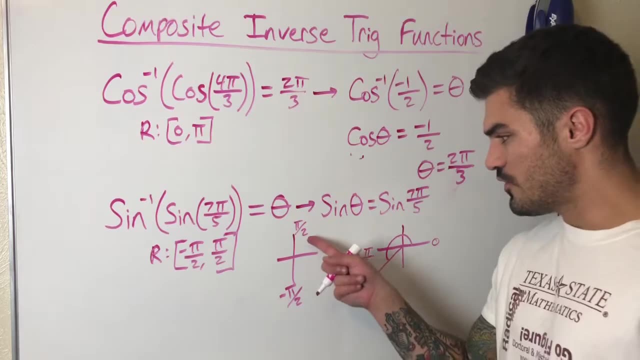 that has a reference angle of 2 pi over 5, and that gives me what? Well, I'm in the third quadrant, so this is going to be negative. So that gives me a negative. So what can I do? Well, first or fourth quadrant. 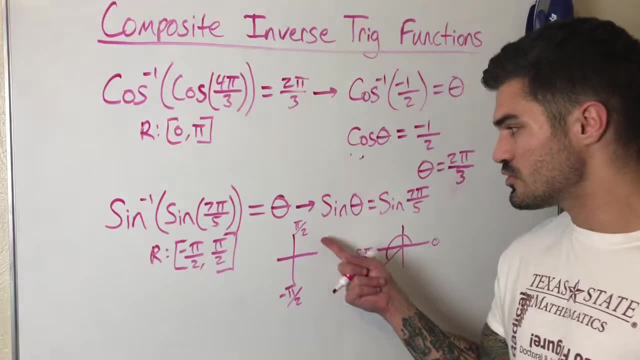 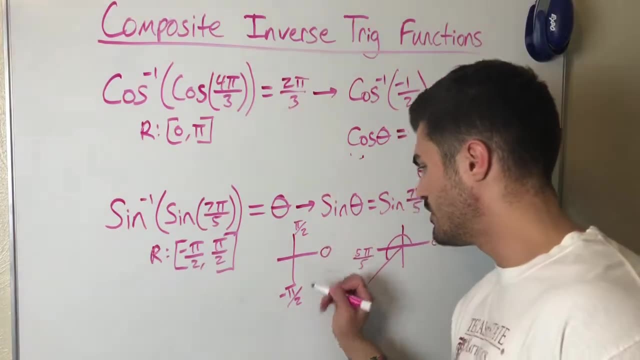 those are my two options. Fourth quadrant gives me negative. First quadrant gives me positive. So I know that this theta is within this fourth quadrant. so it's between negative pi over 2 and 0.. So what is in this quadrant with a reference angle of 2 pi over 5?? 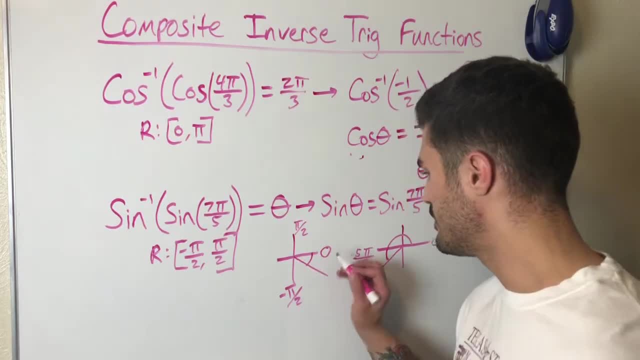 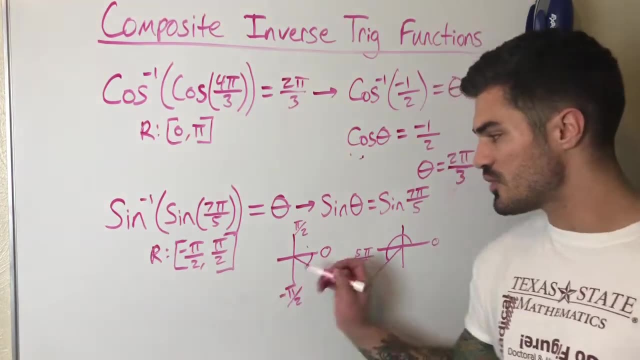 That is negative 2 pi over 5.. Okay, that's that angle. there I'm working backwards. And remember we don't start here and go all the way around to the fourth quadrant With sine inverse. we have to work backwards and work forwards. 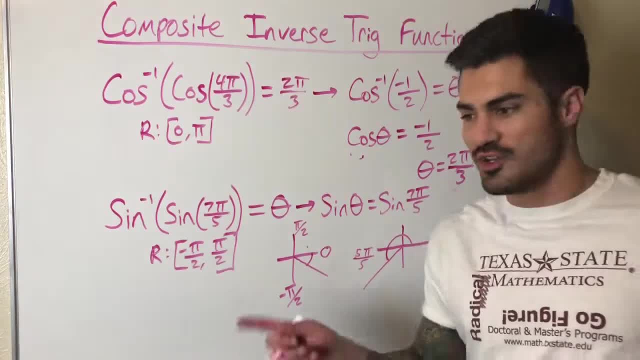 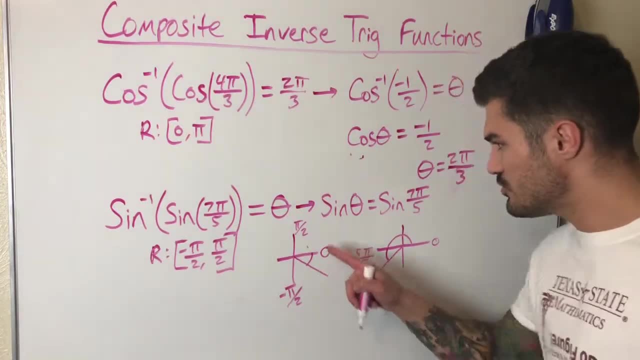 So that's a very common mistake. Students will say, oh, fourth quadrant? and they'll wrap all the way around: No, you want to work backwards. That's how the inverse range works, right. So what is our solution? Well, theta equals negative 2 pi over 5.. 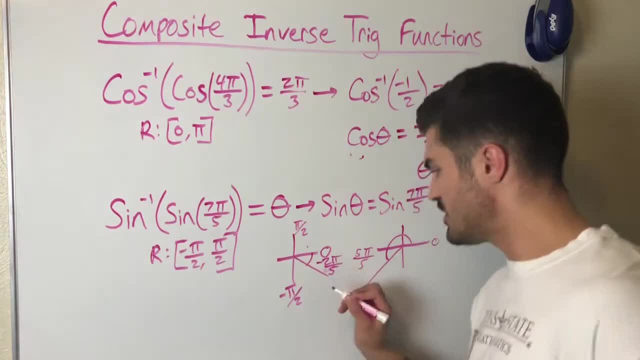 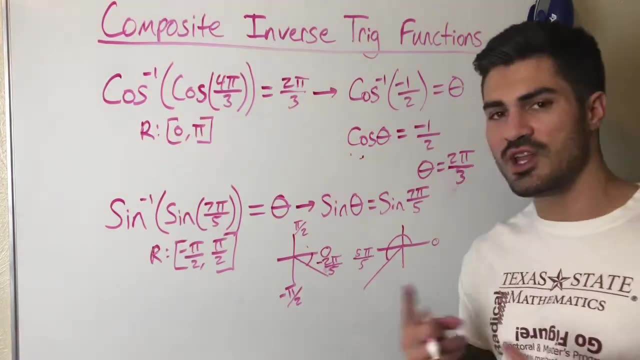 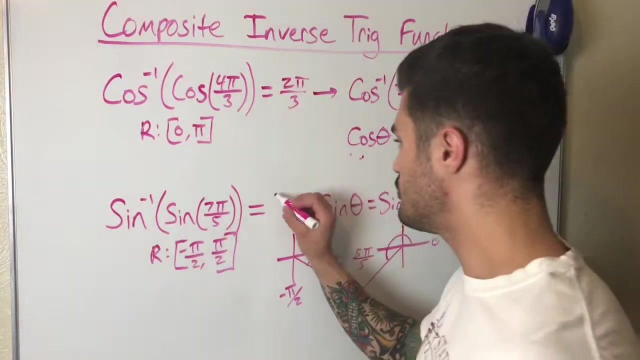 Negative: 2 pi over 5.. So the key to really understanding this is being able to draw angles in standard position, being able to find reference angles and understand what they mean, and knowing what trig functions are positive and negative in which quadrant. So here I have negative 2 pi over 5.. 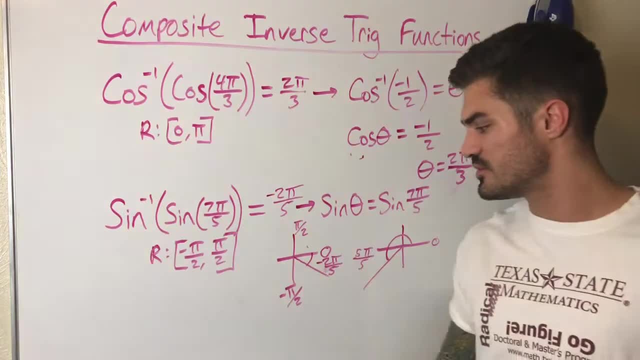 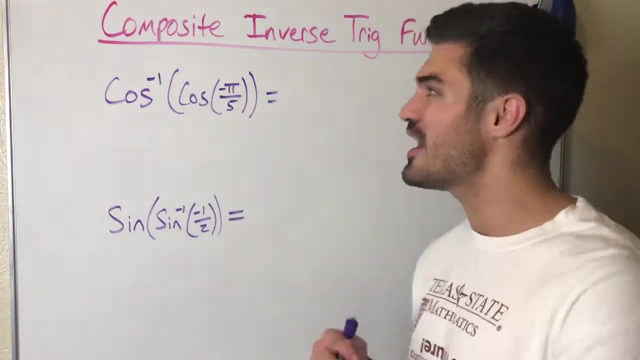 And let's get to a couple more examples and see some more problems. All right, so here's a couple more examples to finish up the video. I will be making a part two with more examples, so stay tuned for that. They'll be harder examples. 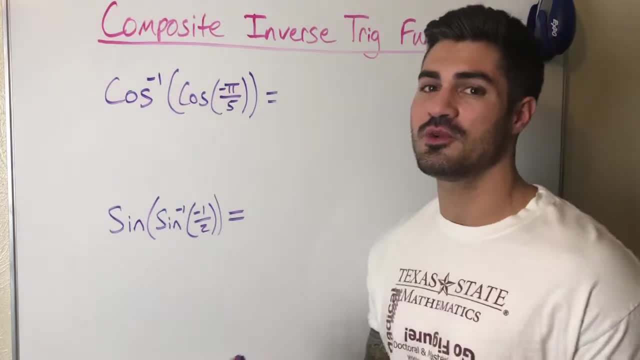 For these. I encourage you to actually pause the video and try them on your own. If you get stuck or you want to check your answer, press play. So by now, hopefully, you pressed play and you have both these answers. Let's go ahead and do it. 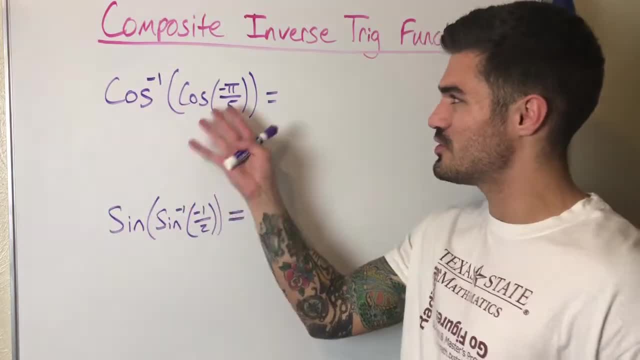 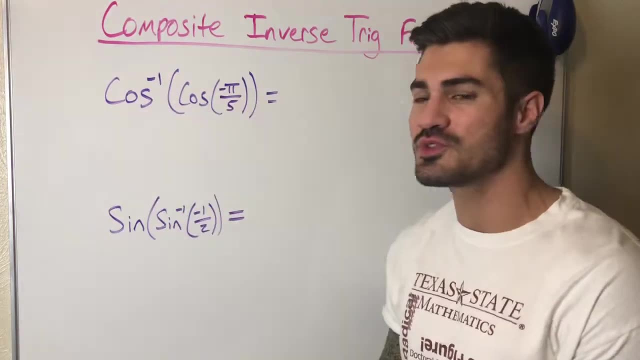 Let's look at this Cosine inverse. that's our outer function. Our inner function is 1.. Our outer function is cosine of negative pi over 5.. So what's the first thing I always do is check to see if this angle is in the range of cosine inverse. 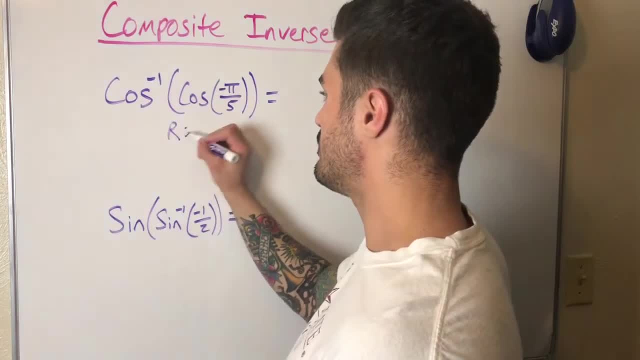 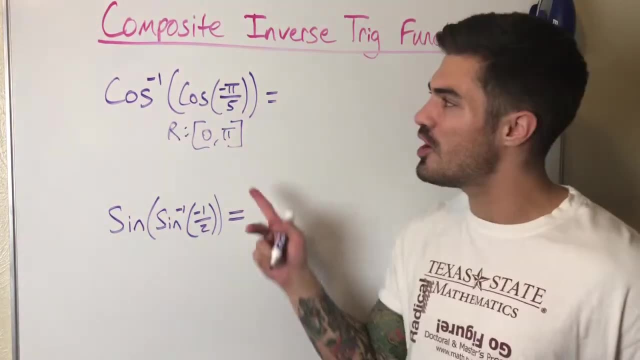 So what is the range of cosine inverse? The range of cosine inverse is 0 to pi. okay, So this is clearly not between 0 and pi. So what's our second step? Well, we look to see if this is on the unit circle. 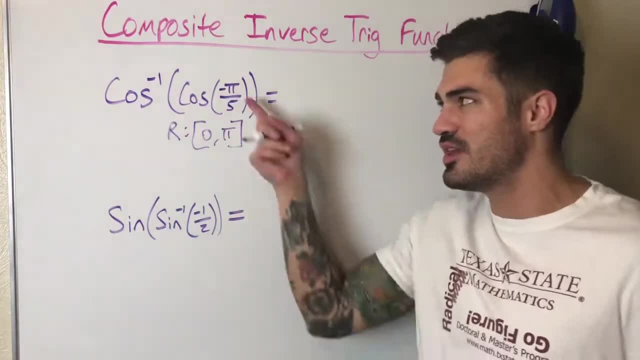 If it is, we can evaluate this and then get something that's a little easier to deal with. It's not on the unit circle. So now, what do we have to do? Well, we know we're going to get some angle out here. 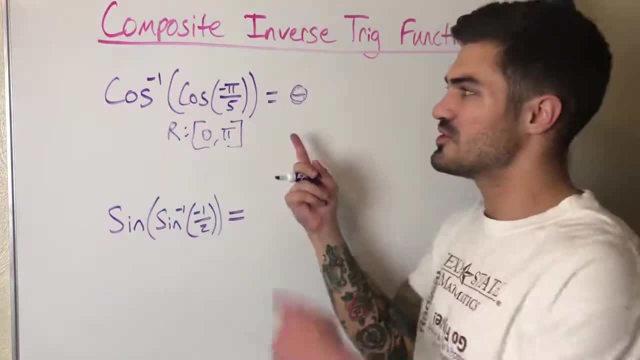 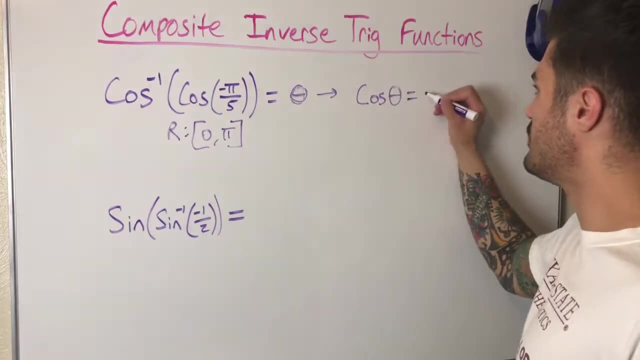 so I can write equals theta and then I can use what I know about inverse functions to switch this input and this output right. So I'll draw an arrow here, and I know that this is like saying: cosine of what angle equals cosine of negative pi over 5, right. 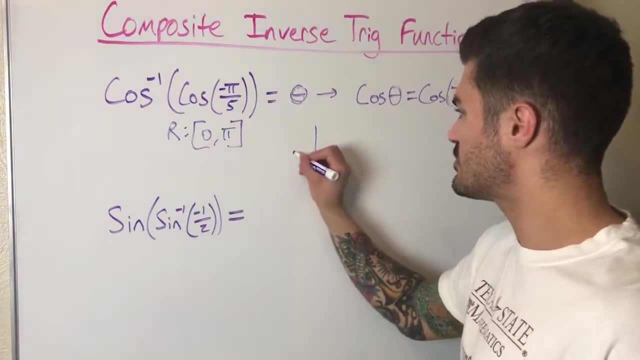 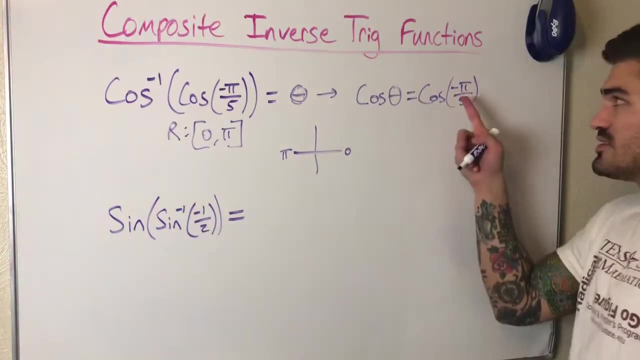 So what I'm going to do is consider my range. I'll draw a little sketch of that: 0 to pi. So whatever this theta is, it's either in quadrant 1 or 2.. So now let me look at this angle: negative pi over 5.. 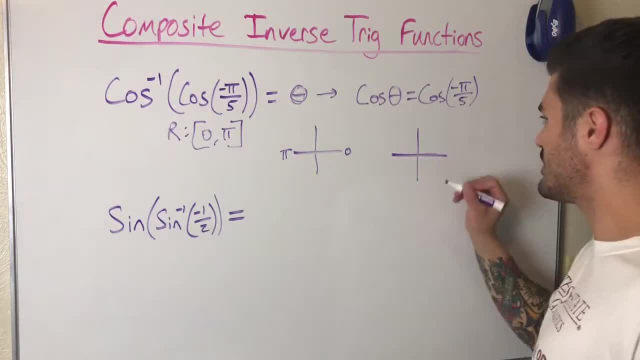 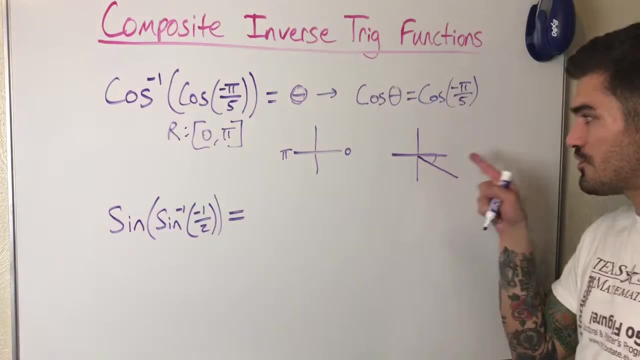 I'll draw a sketch. I always draw as many pictures as I can. It really does help. Negative pi over 5,. I'm starting here and I'm working backwards. My reference angle is pi over 5.. I'm in the fourth quadrant, so I know this is a positive value. 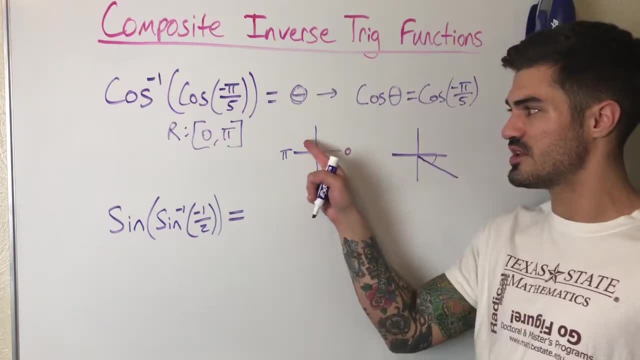 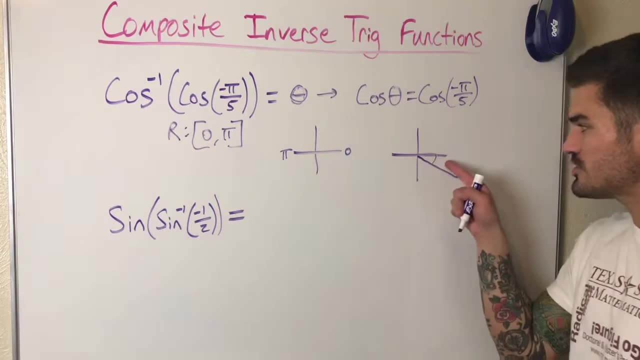 So, since this is a positive value, I'm going to be in the first quadrant, because cosine is positive in the first quadrant and negative in the second quadrant, So I've narrowed it down to first quadrant. So I'm in the first quadrant with a reference angle of pi over 5.. 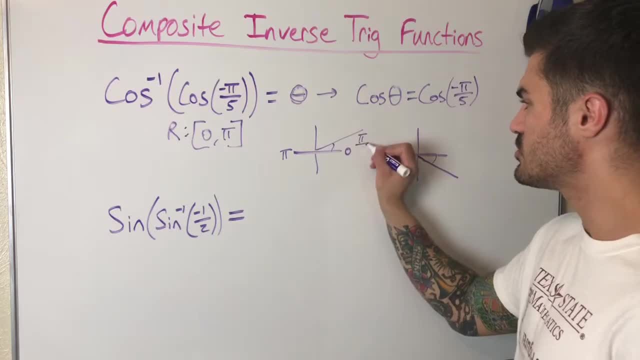 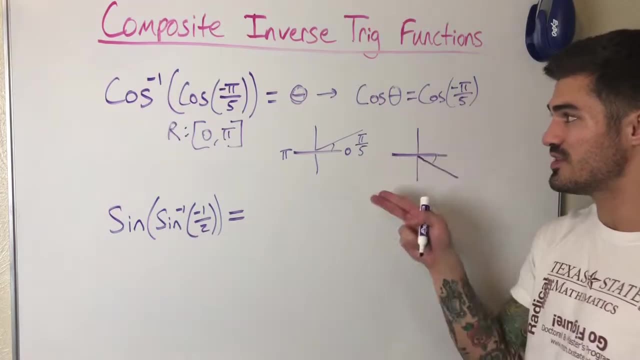 That's simply just pi over 5.. Okay, So what are the two main things I look for? Reference angle and positive or negative, right The sine. So those are the two main things I'm using to get my theta. So in this case I have pi over 5.. 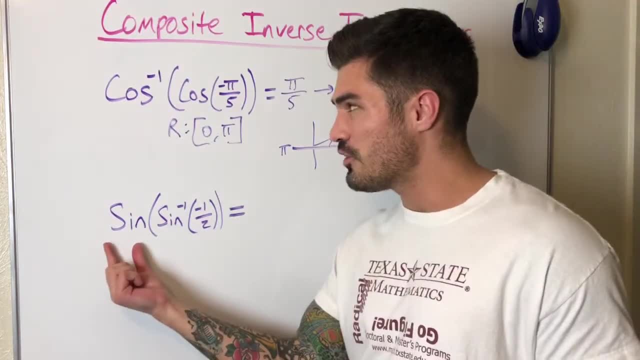 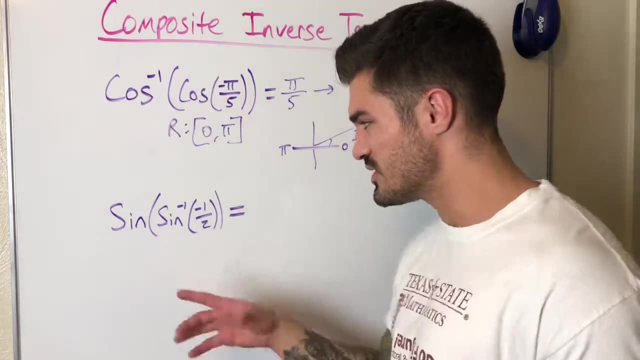 All right. So for this last example it's a little different, because our outer function is no longer an inverse function. We just have regular old sine out here, right, Our inner function is the inverse function now. So it's a little bit different, because out here, 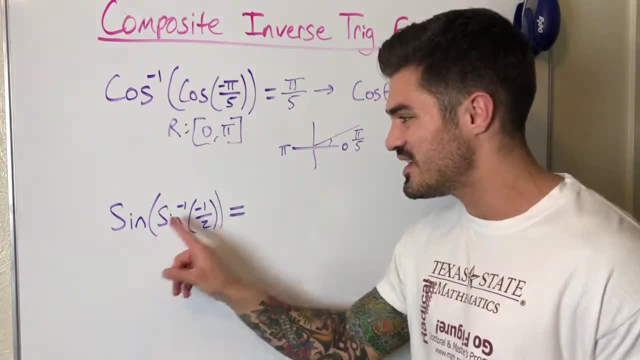 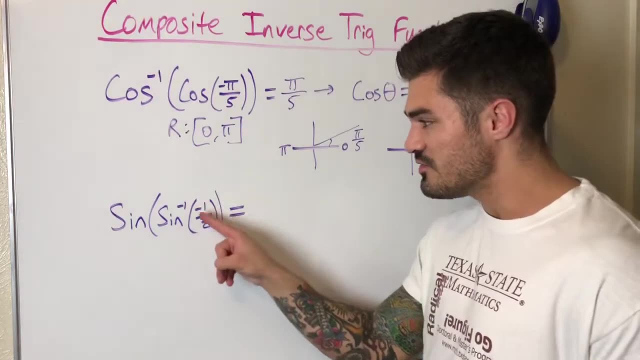 we're not getting an angle anymore, It's just a value, Because sine takes in an angle and spits out a value. Sine inverse takes in a value and spits out an angle. So this sine inverse is taking in this negative 1 half. 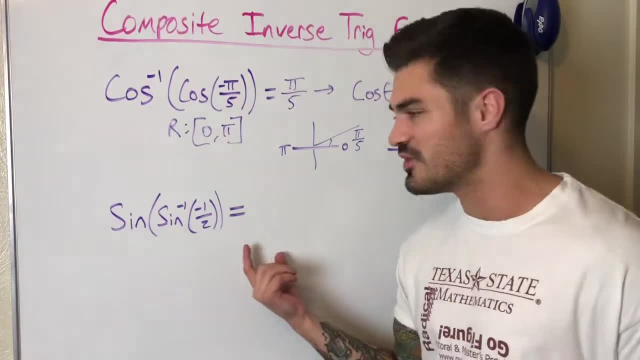 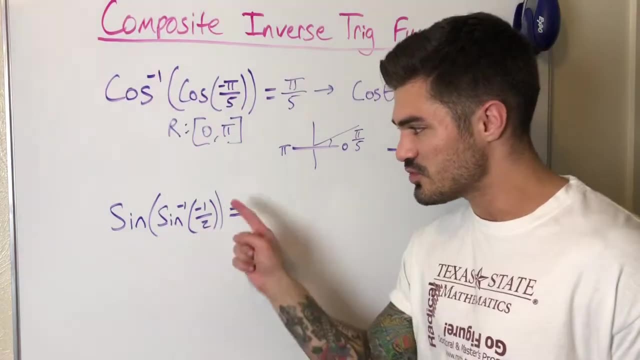 It's going to spit out an angle, Then I'm going to take the sine of that angle right. So what I can really do is start from the inside and work out. I can find what this angle is, replace sine inverse with that angle. 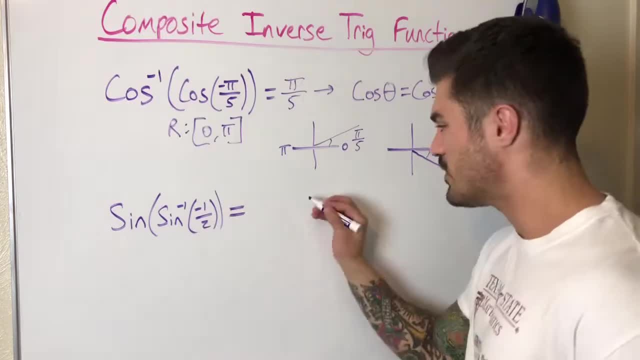 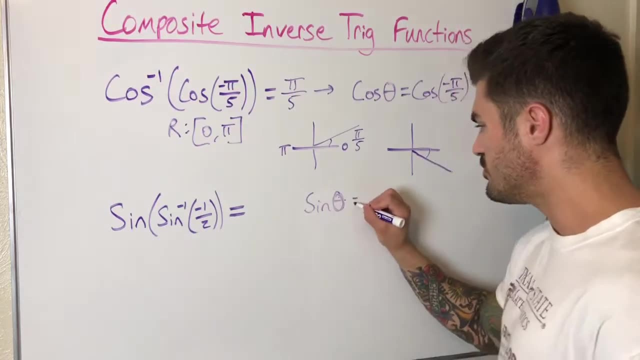 and then take the sine of that angle. So that's what I'm going to go ahead and do. So sine inverse of negative 1 half is like saying sine of what angle? Oh, my marker's dying on me. Sine of what angle equals negative 1 half. 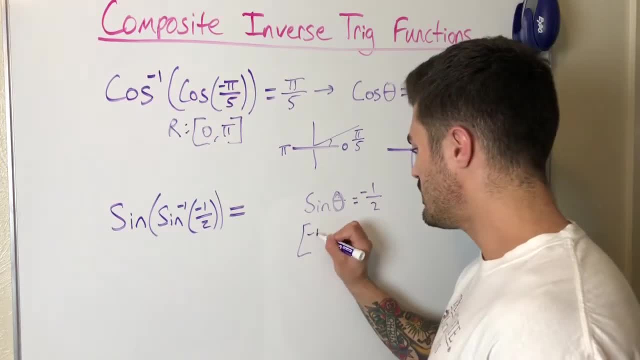 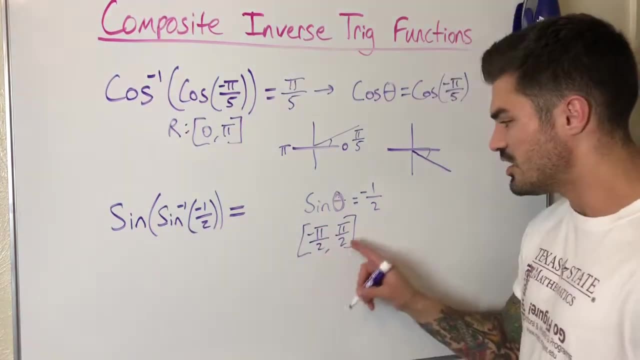 But the problem is my theta has to be between negative pi over 2 and pi over 2.. So I just make sure I stay within that range of sine inverse, So negative pi over 2 and pi over 2.. And since sine is negative, I know I'm going to be in the fourth quadrant. 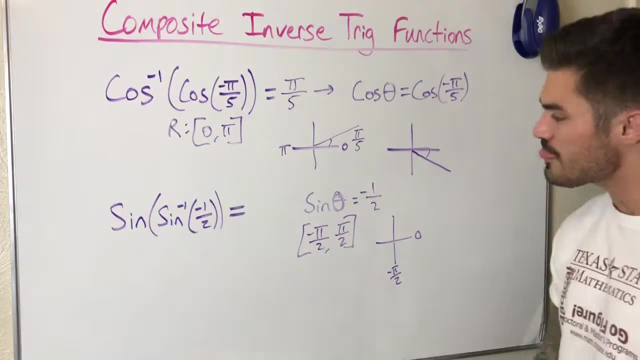 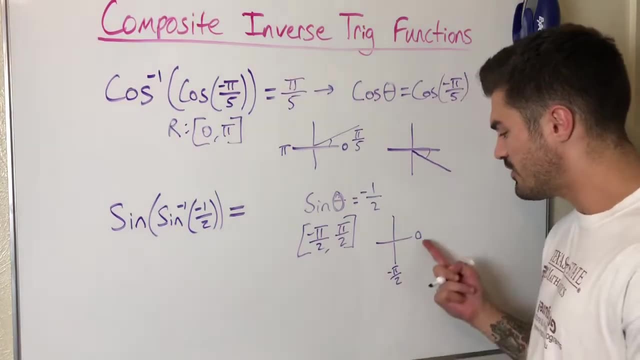 between negative pi over 2 and 0,. right, Let's see. A reference angle of pi over 6 gives me these 1 halves I'm looking for And since I'm between negative pi over 2, I'm going to be in the 4th quadrant. 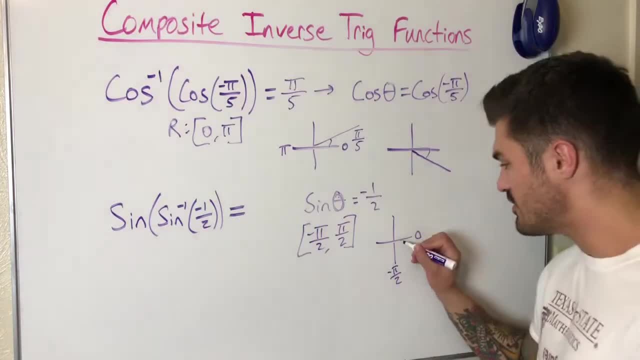 So I'm going to be in the 4th quadrant And since I'm between negative pi over 2 and 0, right and 0, with the reference angle of pi over 6, that means I'm starting here at 0, working backward to pi over 6, which gives me negative pi over 6 for theta. so 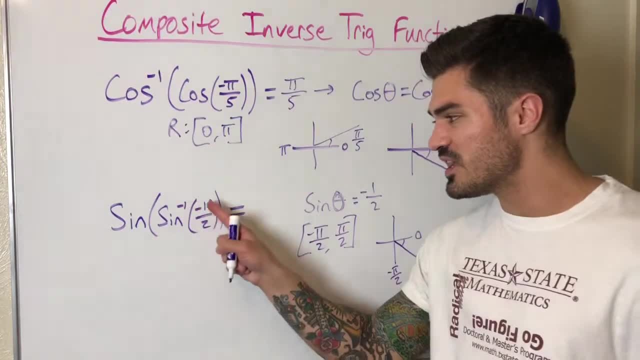 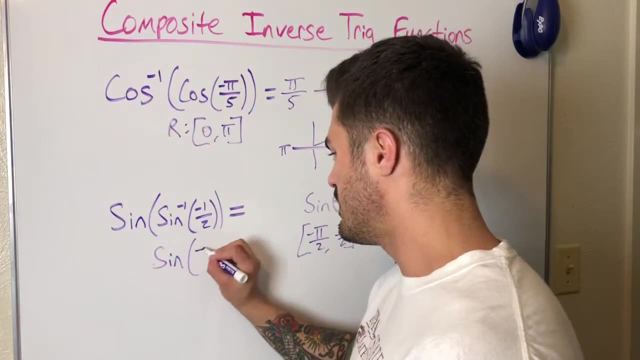 this theta is negative pi over 6, which means sine inverse of negative 1 half is negative pi over 6, which means I can replace this with negative pi over 6, so I have sine of negative pi over 6, which equals what that equals negative 1 half. 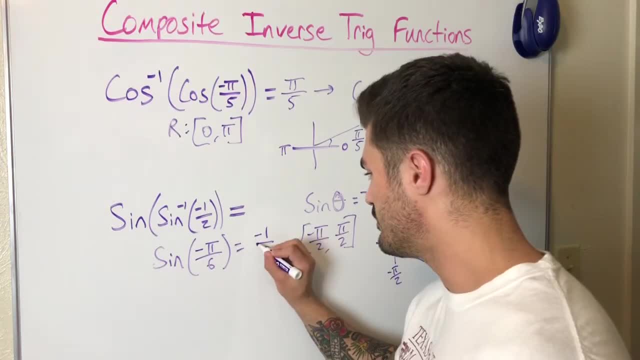 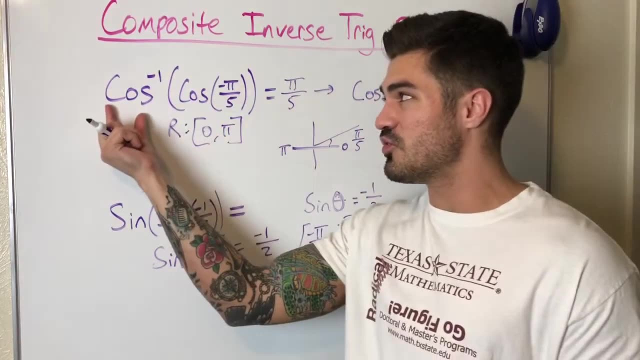 right. so do we notice a pattern here? yes, there is actually a shortcut. there is a shortcut. I can, in this case, just cross these out. right, I couldn't in this case, because I had to make sure it's within the range of inverse sine. okay, but our 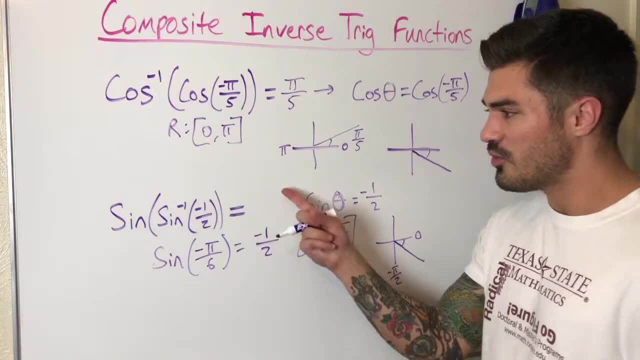 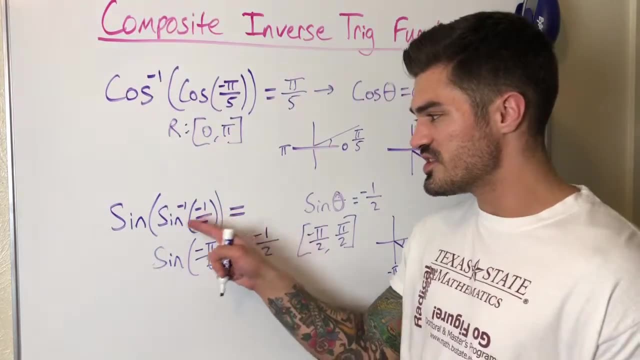 range of sine is not restricted, right, our range of sine. that just gives us values. okay, so in this case we're not really too worried. all we have to do is make sure that whatever is inside this sine inverse right, this inner function, that whatever is inside here is obviously 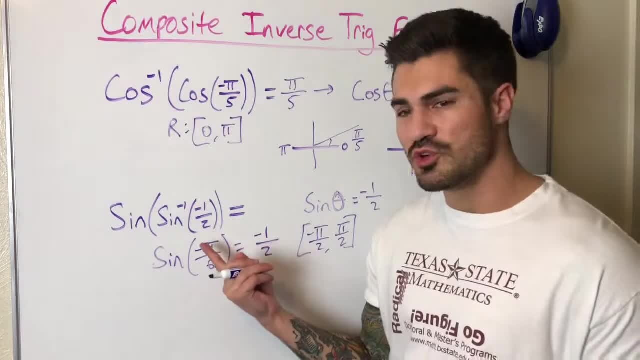 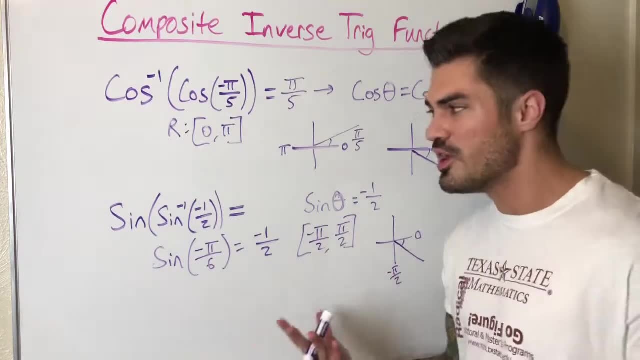 in the domain of sine inverse. so if I had like negative 2 or something in here, then I'd rewrite it as sine theta equals negative 2, which is never possible. so if we have something like that, then we have no solution, but other than that we can.